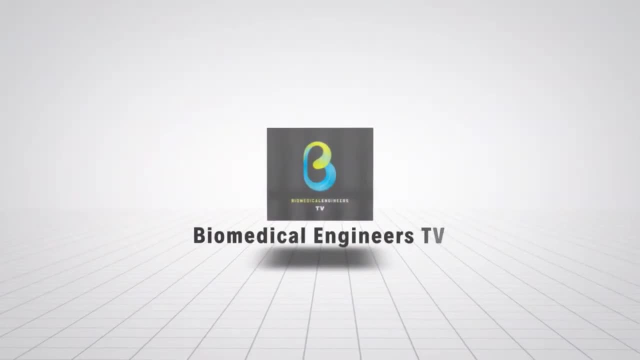 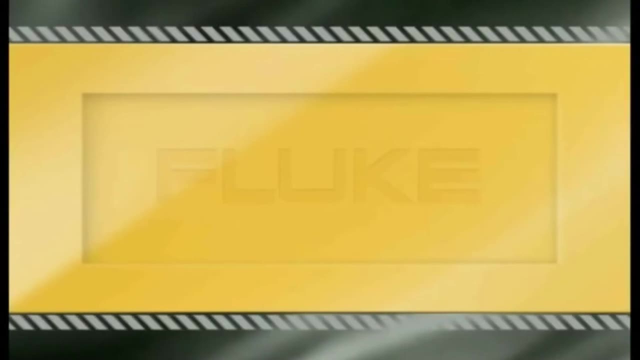 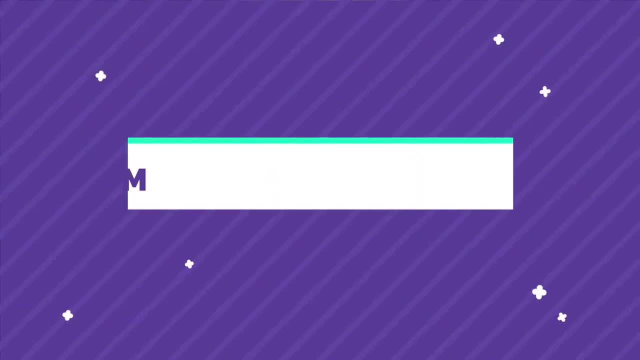 Welcome to the Biomedical Engineers TV. If you are watching this video first time, I encourage you to begin with the first part of this video to understand the electrical safety standards of medical equipments. In this last video we will cover up the medical equipment type. 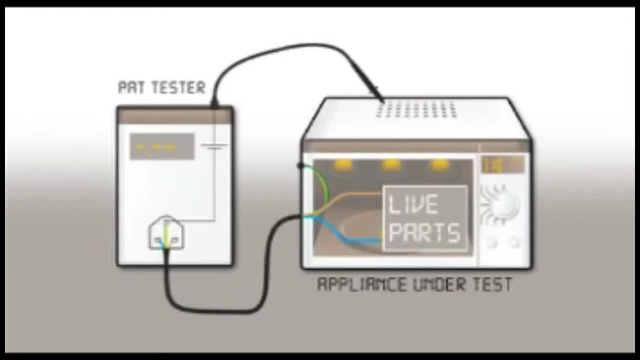 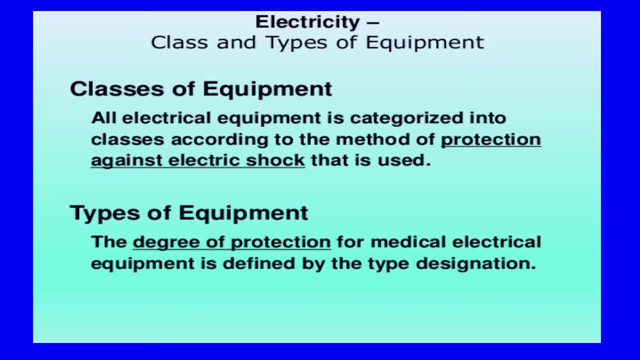 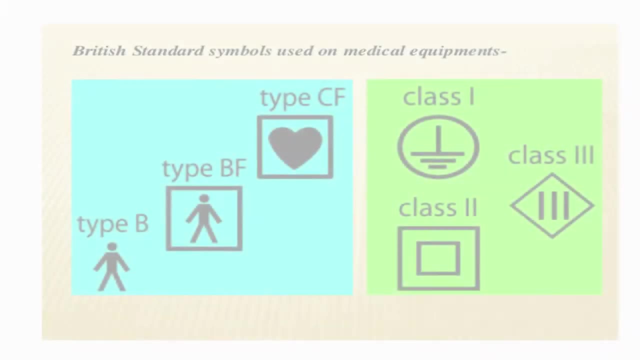 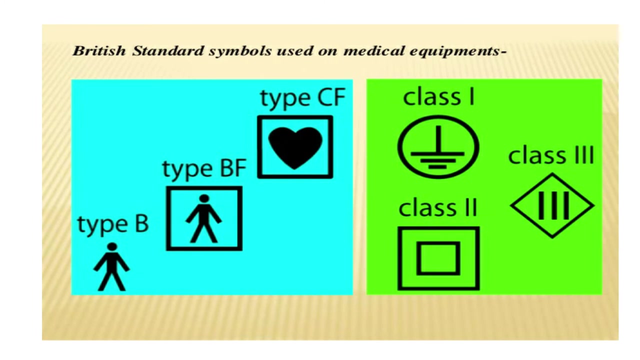 The class of equipment defines the method of protection against electric shock. The degree of protection for medical electrical equipment is defined by the type designation. The reason for the existence of type designations is that different pieces of medical electrical equipment have different areas of application and therefore different electrical safety requirements. 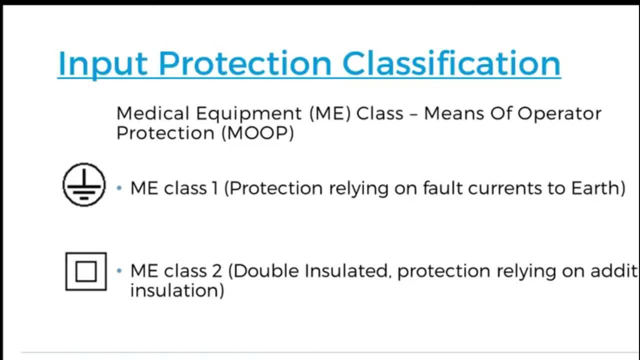 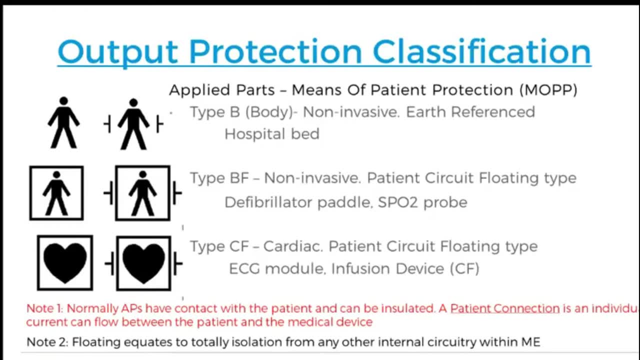 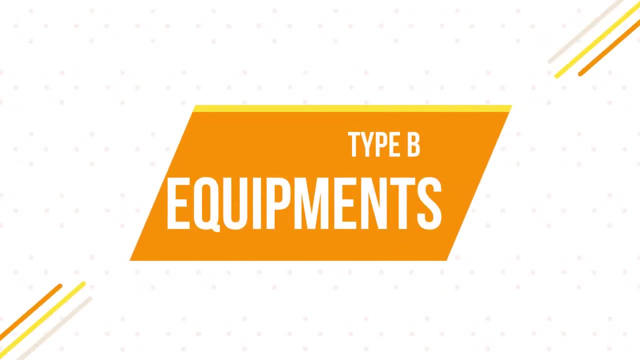 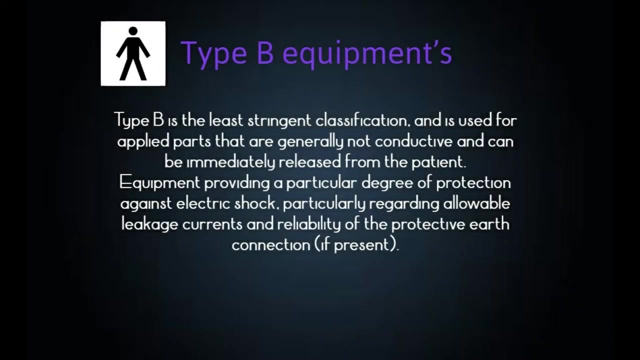 For example, it would not be necessary to make a particular piece of medical electrical equipment safe enough for direct cardiac connection if there is no possibility of this situation arising. Let's begin know about type B equipments. Type B is the least stringent classification and is used for applied parts that are generally not conductive and can be immediately released from the patient. 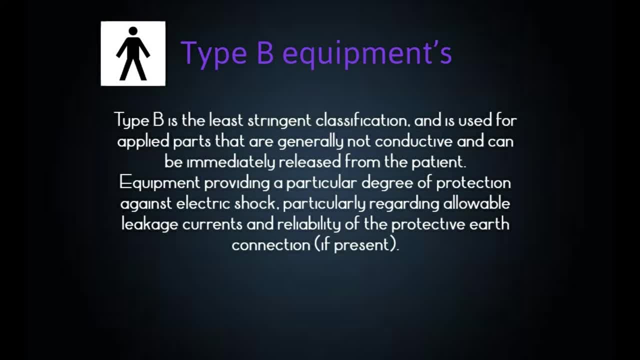 Equipment providing a particular degree of protection against electric shock is called a type B equipment. Equipment providing a particular degree of protection against electric shock is called a type B equipment. Equipment providing a particular degree of protection against electric shock is called a type B equipment. 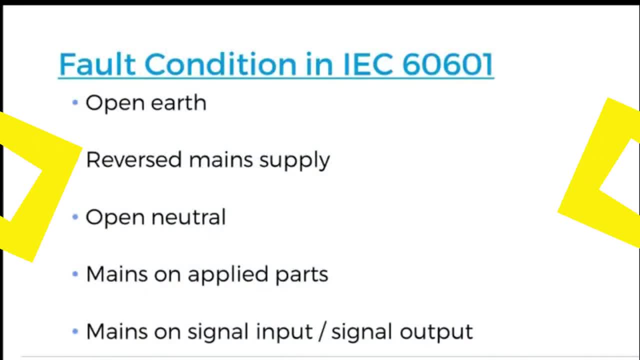 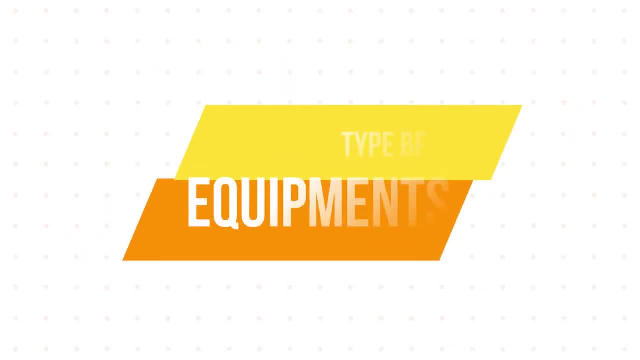 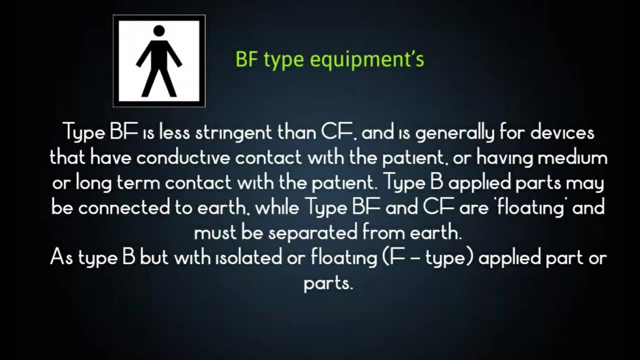 In this video we will look at the four major types for electric shock. in general, This is due to the number of applications by electrical equipment that the diagnosis of primary length of electrical current can attempt to obtain. When we determine series of cases of principal ableże, use a department and say that the Breath code may be almost叫 SoI Am-when there is noな. 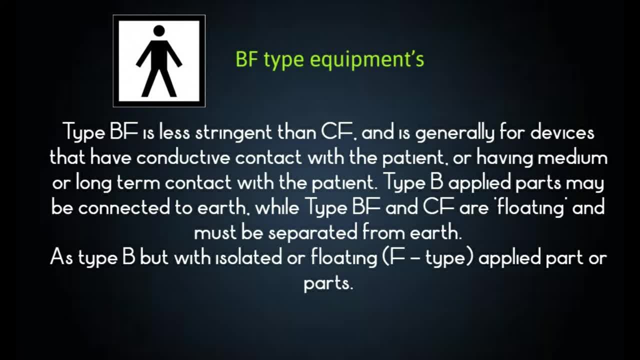 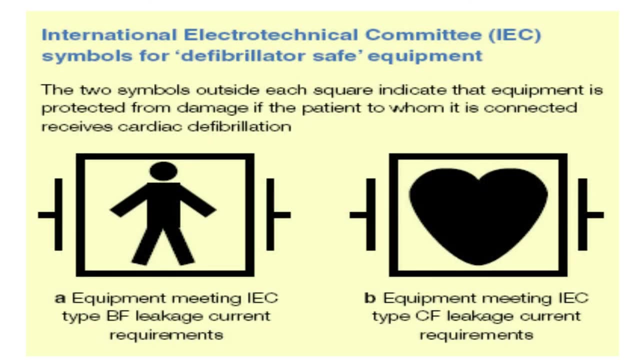 is one group of 5 versus 3 equal spokes In this lack of a discreteized set of web, web otta, or You have to believe that there is no force, while type BF and CF are floating and must be separated from Earth as type B, but with isolated or floating F-type applied part or parts. 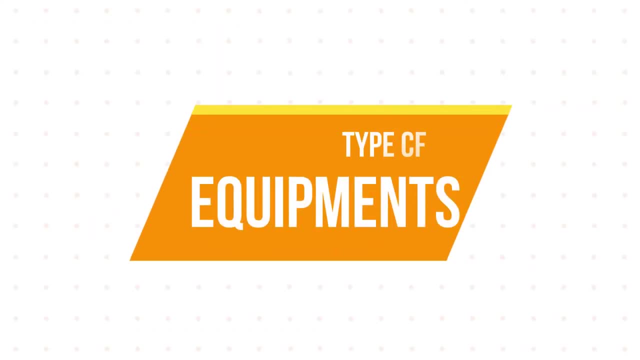 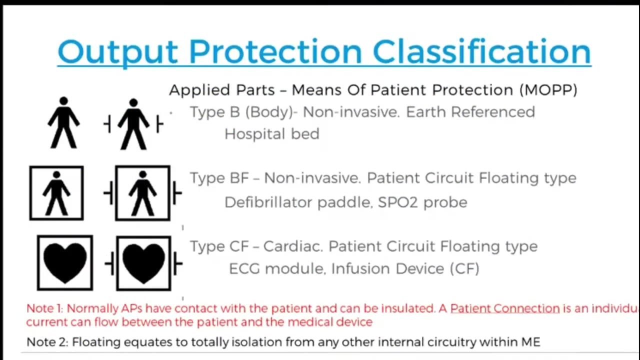 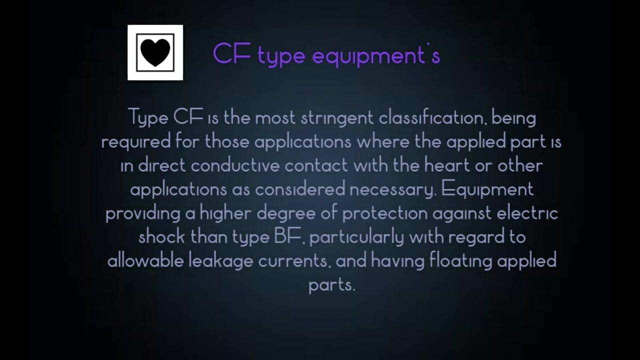 And the last one is the CF type equipments. Type CF is the most stringent classification being required for those applications where the applied part is in direct conductive contact with a heart or other applications as considered necessary. Equipment providing a higher degree of protection against electric shock than type BF.